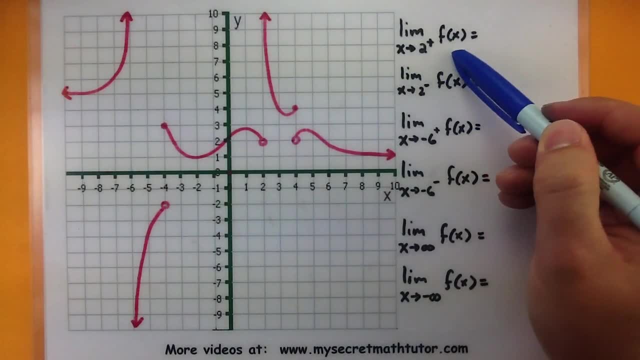 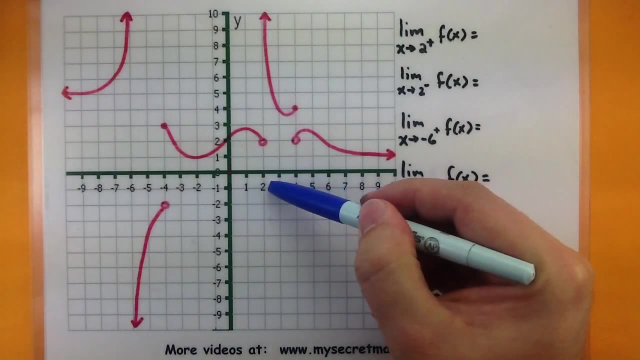 says: what is the limit as x approaches 2 from the right of our function? Okay, so let's find 2 on our x-axis. Here we are and we're approaching 2 from the right side. Well, if we look at our function as we're approaching 2, notice how it just gives us a little bit. 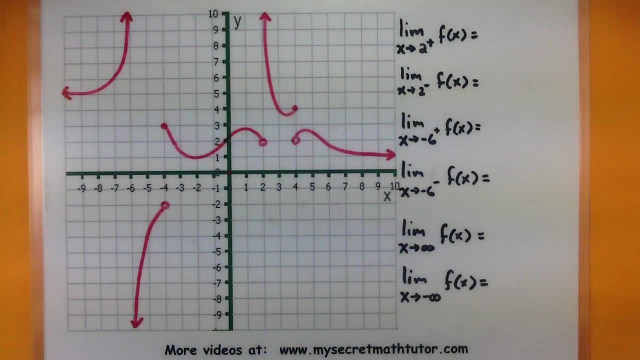 of space. It's arbitrarily large. It just keeps going up and up and up. So this is an indication that the limit would be at infinity. All right Now, just because it's approaching infinity as we go from 2 on the right side doesn't mean that that also has to happen. 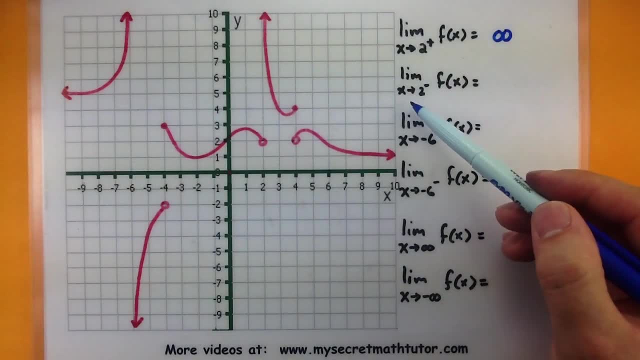 on the left side. In fact, look at the next one: The limit as x approaches 2 from the left. Well, as we're going on the left side, this just simply wants to approach the value of 2.. So it is possible to get an infinity on one side and not on the other. All right, let's. 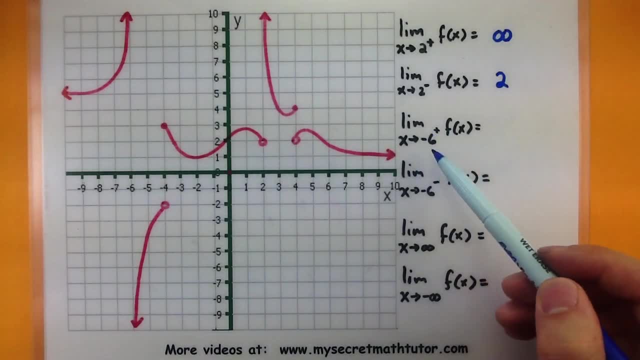 do some more. This next one says the limit as x approaches negative 6 from the right side. Here's our negative 6.. We're approaching from the right side and now we can see that our function is getting large but negative. So this one is going towards negative infinity. 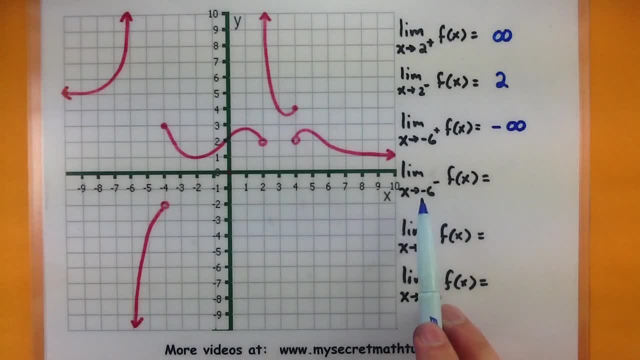 Okay, looking good, Let's go ahead and approach x. Let's have x approach. negative 6 from the left side. So here's our negative 6 again. As we go from the left side, now we're just getting really large, So that one goes towards infinity. All right, So notice how in these 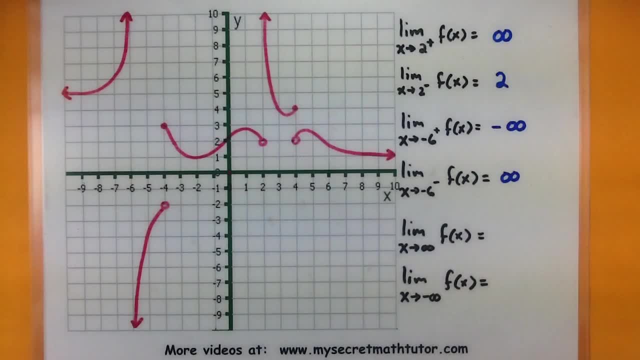 ones. x was always approaching some sort of number, and we're either doing it from the left or right side. In these last two, x will be approaching infinity or x will be approaching a negative infinity. So imagine going down that x axis all the way down to infinity, or 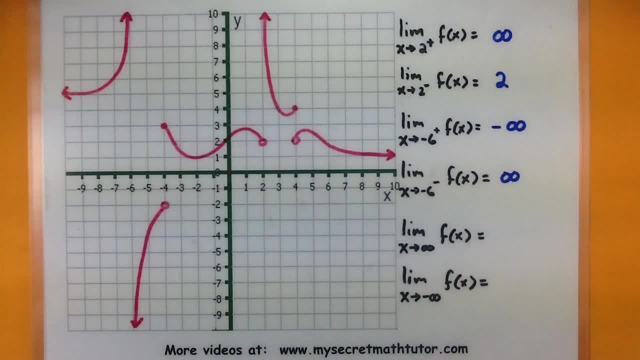 approaching negative infinity again along the x-axis. All right, so what is happening as x goes towards infinity? Well, our function does a lot of crazy things, but as we get down here and imagine, you know, continuing on into infinity, it looks like it just wants to be the value of 1.. So we'd say that.